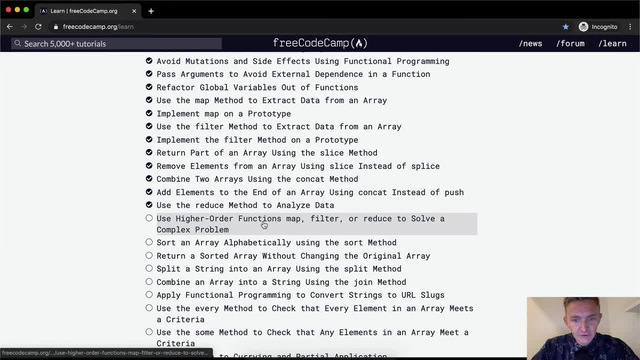 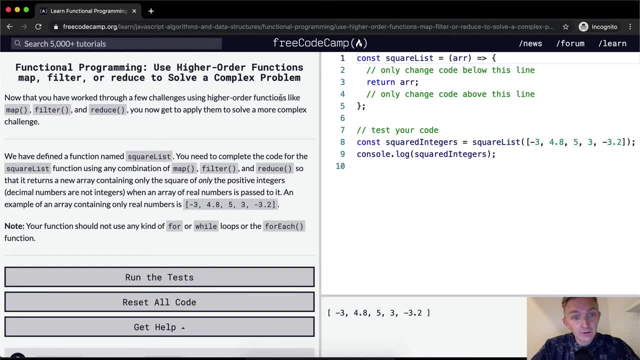 Hello friends, welcome back. Today we're going to use a higher order functions like map, filter or reduce to solve a complex problem. Now that you have worked through a few challenges using higher order functions like map, filter, reduce, you now get to apply them to solve a more complex challenge. 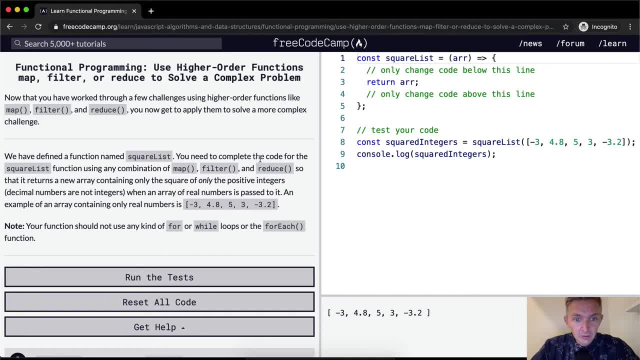 We have defined a function named squareList. You need to complete the code for squareList function using any combination of map filter and reduce so that it returns a new array containing only the square of only the positive integers. Decibel numbers are not integers. 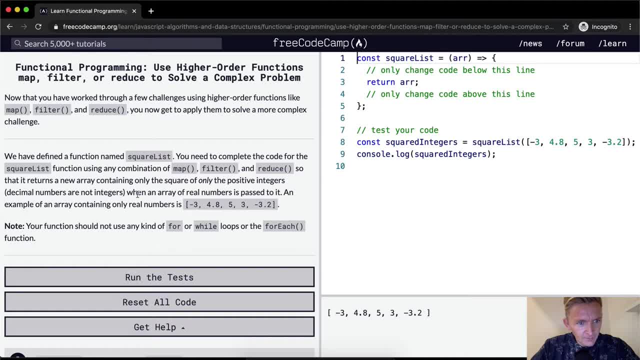 Well, only of only positive integers When an array of real numbers is passed to it. An example of an array containing only real numbers is negative 3, 4.8, is an array with the numbers negative 3, 4.8,. 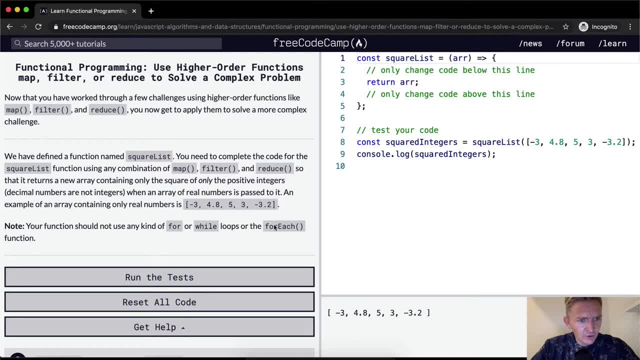 4.8, 4.8, 5,, 4.8,, 5,, 3,, 4.8,, 5,, 3, and negative 3.2.. Your function should not use any kind of for or while loops or the for each function. 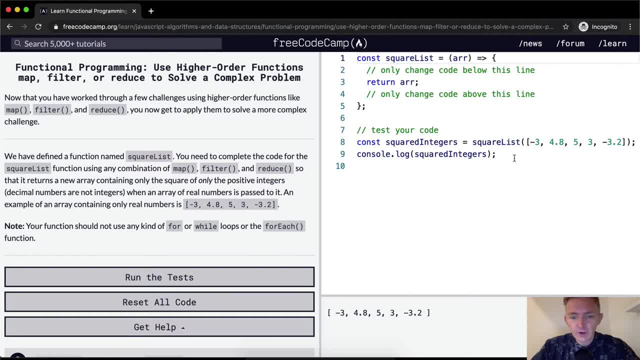 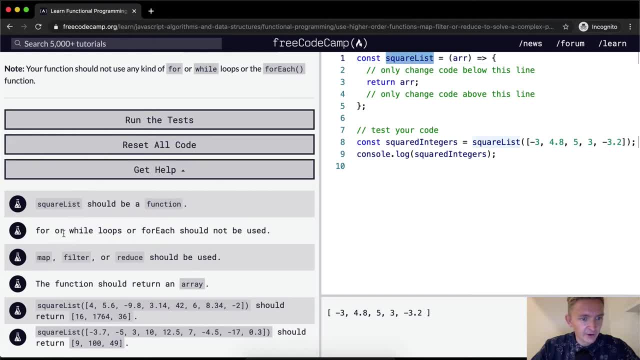 Your function should not use any kind of for or while loops or the for each function Interesting: Okay. so If I look over here it should be a function SquareList. Okay, it's already a function, So I bet that would pass if we ran it now. 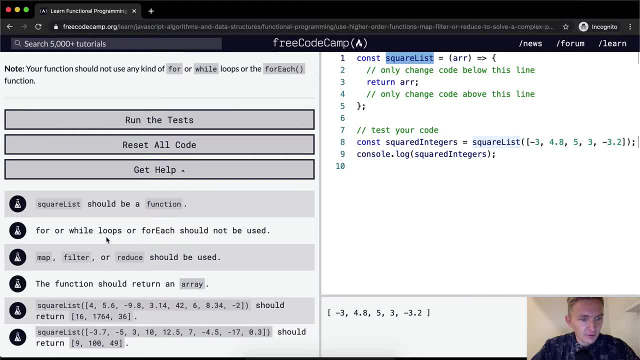 Or This would probably pass, but we're not doing anything. We don't want to use while or for each loops. We should use Oh it says, or So that means that we can use probably one or many. The function should return an order. 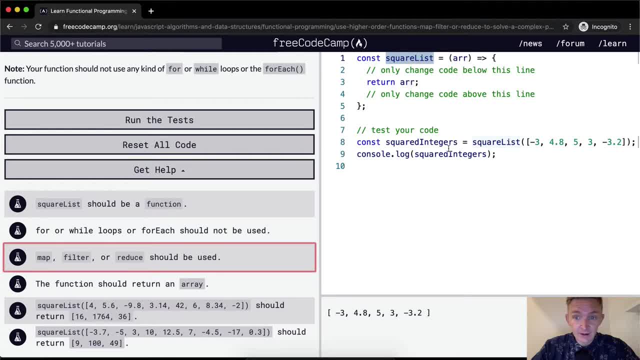 The function should return an array. Look at that. It's not returning an array yet. Well Yeah, SquareList, It's getting passed in an array and it's returning an array, So, And this should return 16.. 174,, 64, and 36.. 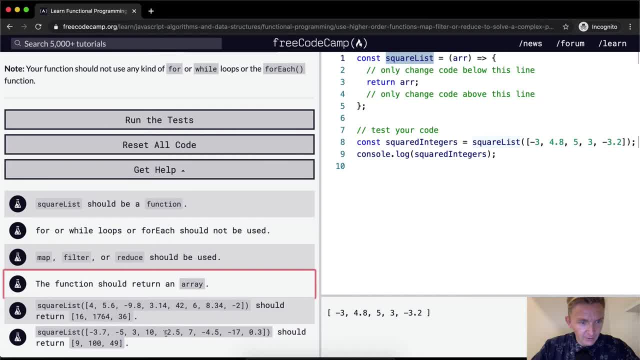 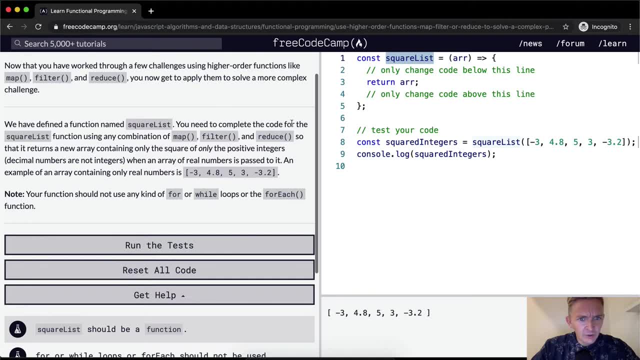 SquareList should return 9, 149.. Okay, so what do we really want it to do? here We have to find a function. You need to complete the code SquareList function using any combination map filter so that it returns a new array containing only the square of only the positive integers. 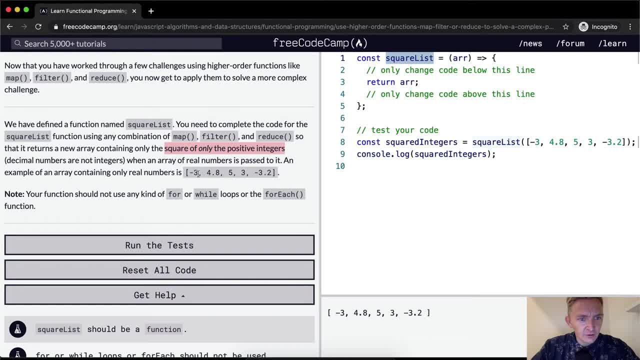 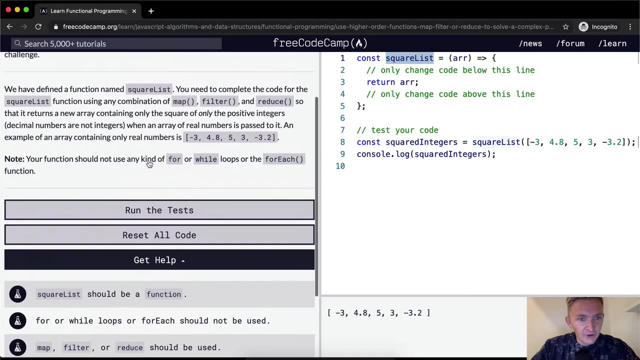 Decimal numbers are not integers when an array of real numbers is passed to it. An example of an array containing: Okay, so this is real numbers, but we want only positive integers. Okay, so the square of positive integers, So the positive integers here. 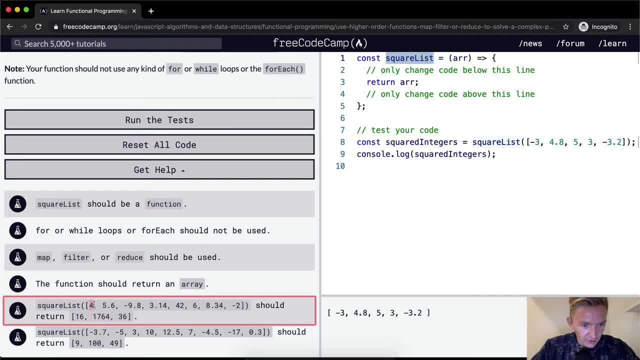 4 is a positive integer. 4 squared, So 4 times 4, is 16.. 4, 8,, 12,, 16.. So that's that one. This is not a positive integer. This is not a positive integer. 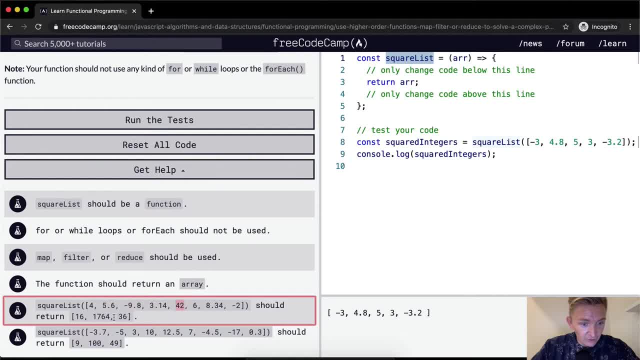 This is not a positive integer. This is 42 times 42.. 1,, 7,, 6,, 4.. Perfect And 6.. So we, first off, we just want to filter the positive integers, And then we want to sum them each up. 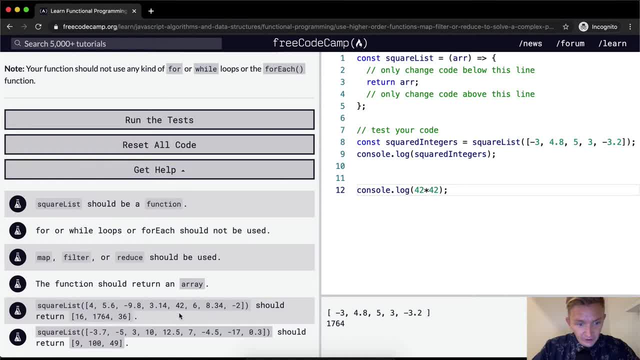 So, yeah, I think that that's a way to go. We want to filter And then we want to map them by squaring them by themselves. So I think that's a pretty straightforward answer to this question. So let's get after it. 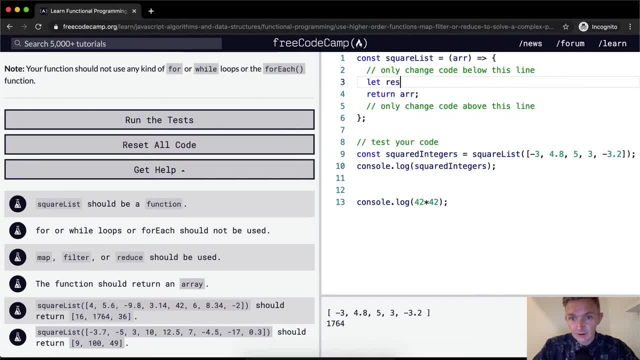 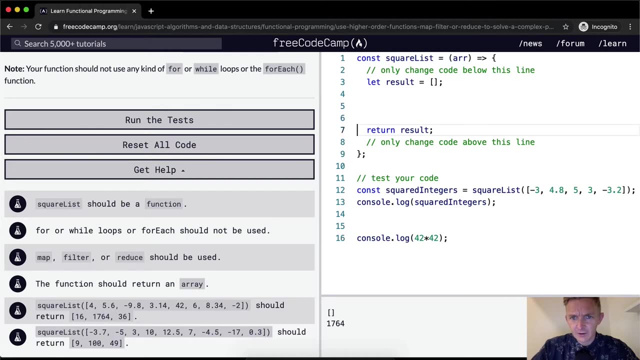 First off, I would say: let's let a result array is equal to here, And then we can return the result. I think that's a good way to start. That way we're not trying to manipulate the array at all, Because that is against our functional programming background. 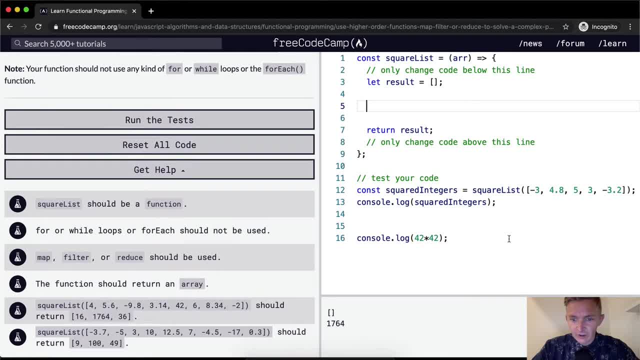 And yeah, so here we can get rid of this now. I was just doing that Because it's good to question assumptions early. Are we getting the square of those? I became clear that that's what we're going for, And that way I was able to figure out what we're trying to do. 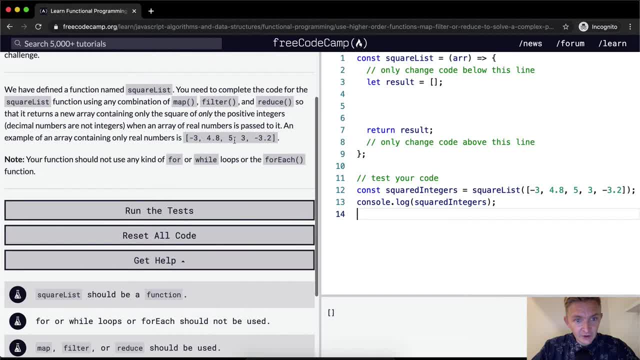 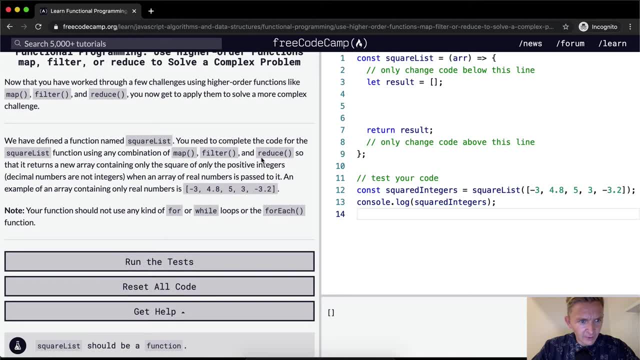 Let's see For this one, a positive integers. I'm pretty sure these are all even, But does it care whether they're even or not? Of all positive integers containing only the square of only the positive integers, Okay, I'm thinking 3 times 3.. 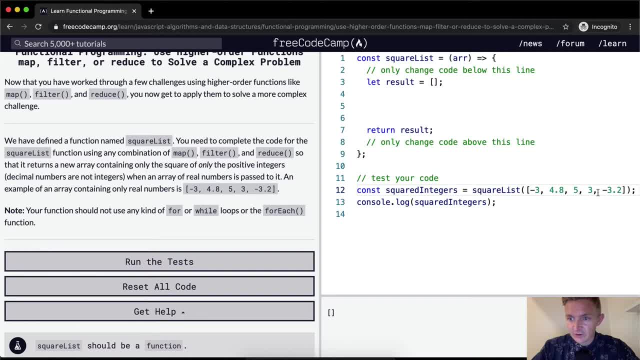 Yeah, 3 squared is 3 times 3 times 3.. So 3, 6, 9.. We basically want our result on this one to be: 5 times 5 is 25.. And 3 times 3 is 9, right. 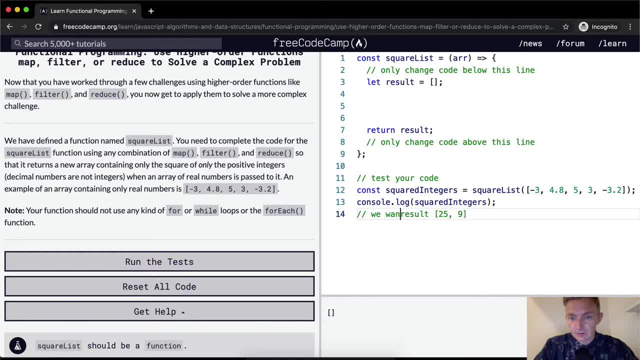 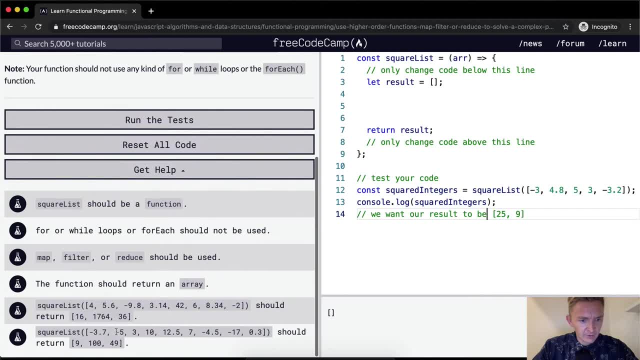 So we want our result to be, Let's see, 3.. Well, instead of just doing this random one that they have here, why don't we do one where we know the answer? So I'm just going to pass this into here. 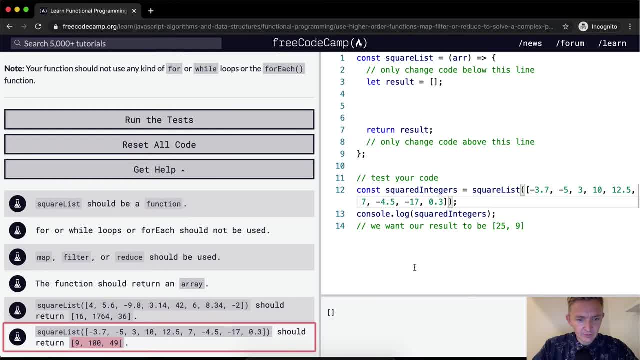 And then we want our result to be this: Yeah, that's an assumption. 7 times 7 is 49. So that's what we want. We want our result to be this: Okay, cool. And so right now, we're just getting an empty array. 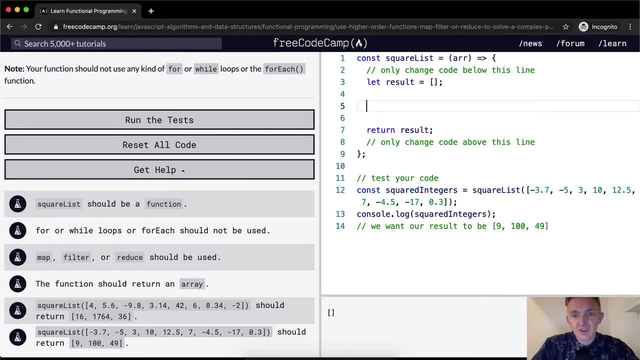 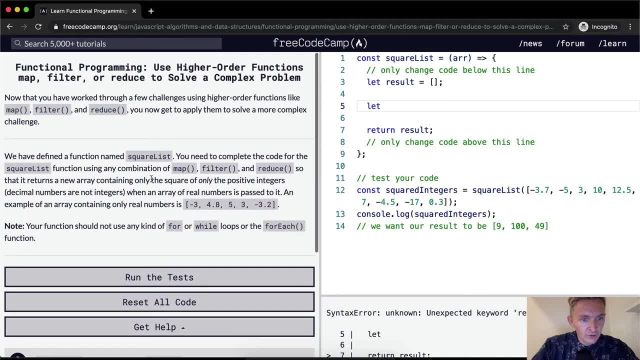 So what do we want to do First? we want to say: Let First off, we want to just get real numbers When an array of real numbers is passing containing only the square of only positive integers. So we want to say: positive integers is equal to what? 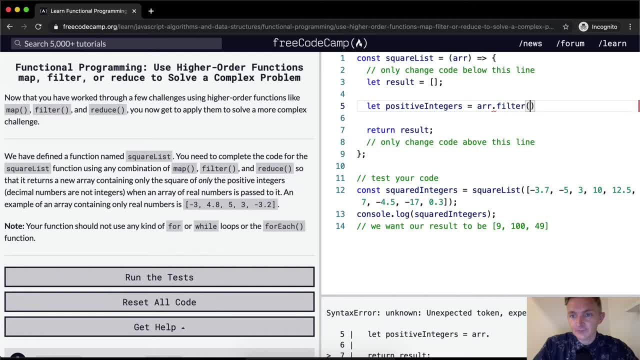 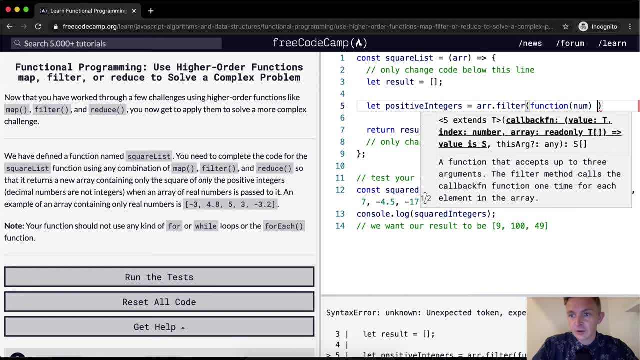 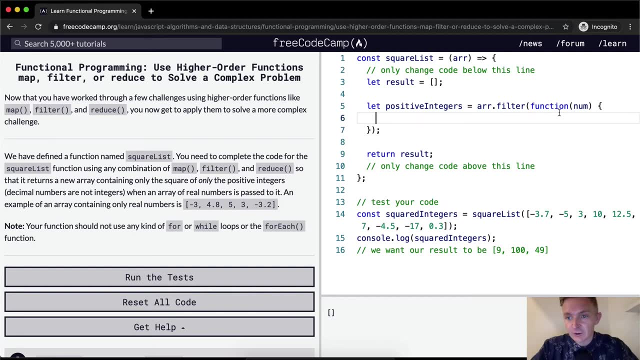 The array dot filter And I'm going to do old JavaScript initially and then we'll refactor later. So this is the older one. So this is the older way of writing the functions And then we'll refactor it to arrow functions later. 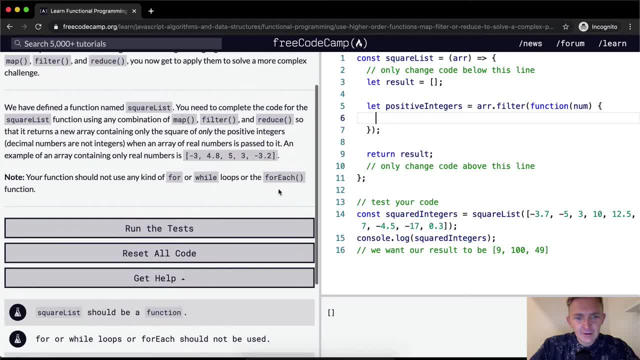 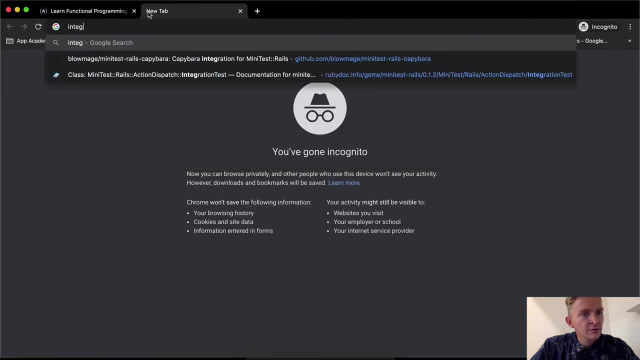 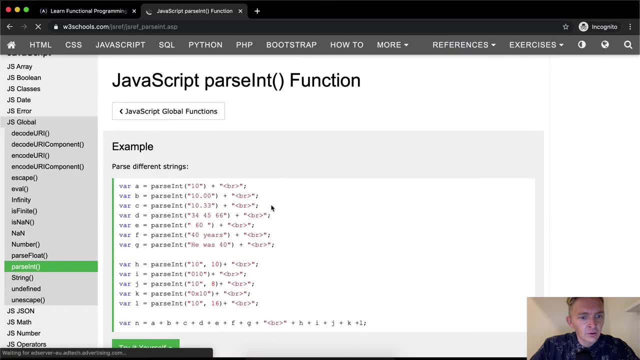 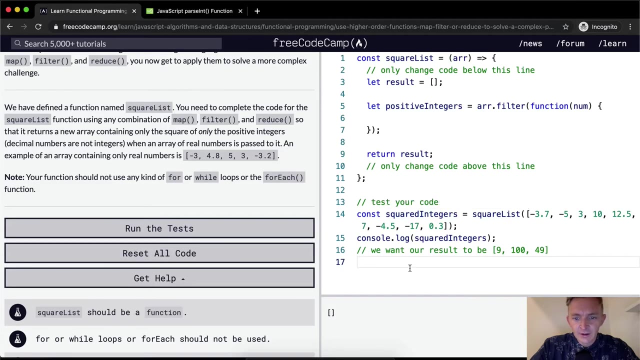 So how do you say that? If num, Let's see Positive integer. I think that we could go like: If my console dot log, Let's say 10.2 is equal to parse int 10.2.. Okay, that's false. 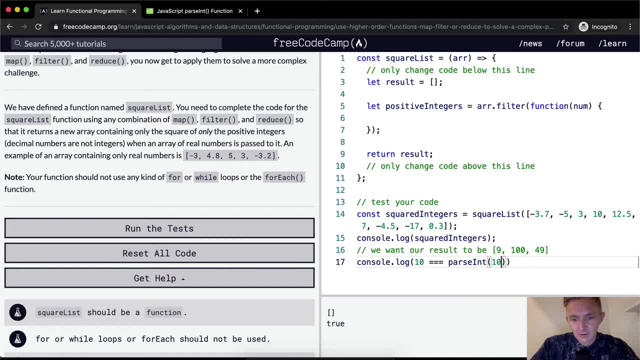 But what if we were to pass in 10? That becomes true. No, but Oh, three, That becomes true as well. So that doesn't work. Hmm, So we want to find a way to find out whether or not. 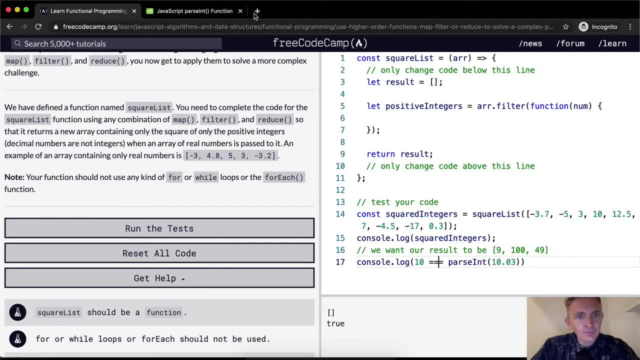 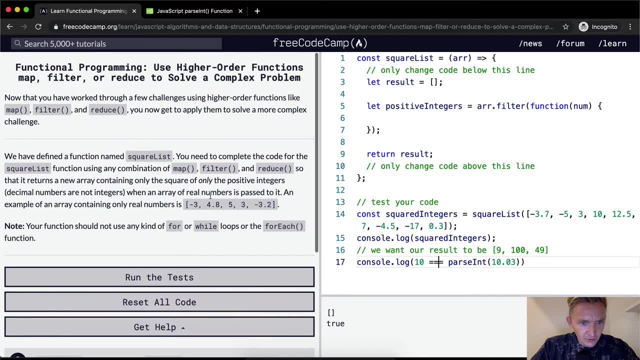 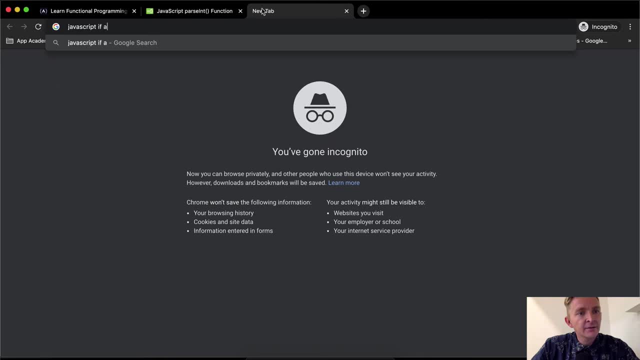 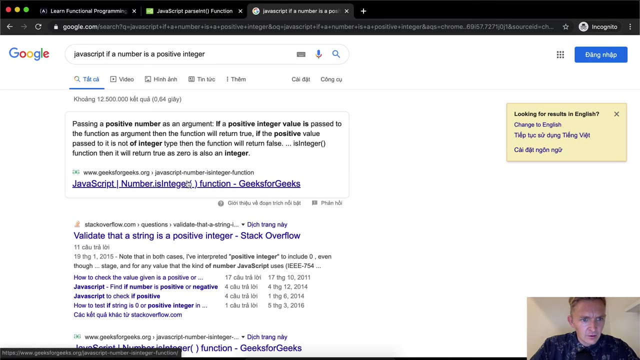 Triple equals parse int. Okay, so what I'm trying to find out is: how do we find JavaScript, How to find out JavaScript? if a number is a positive integer Is integer. Oh cool, Number dot is integer. So could we go? 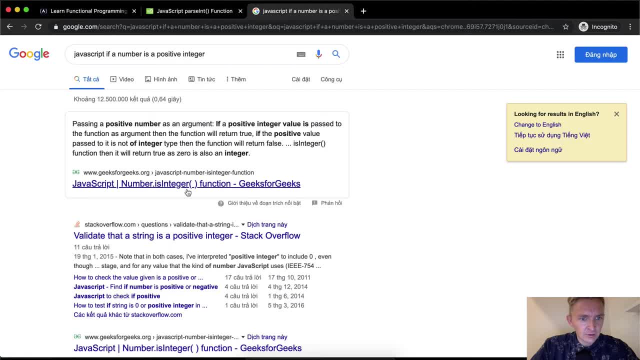 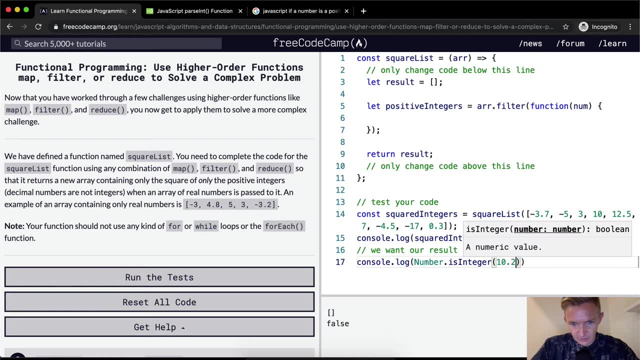 Number dot is integer, And then we could say 10. This should be true, 10.2.. False, Negative, 10. False. Hmm, Well, we know that. Okay, so we could do it two things. Okay. so if 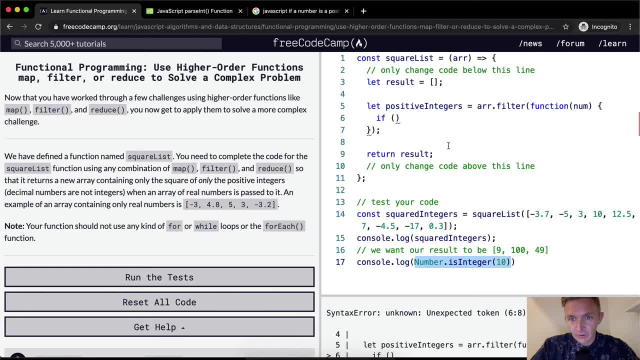 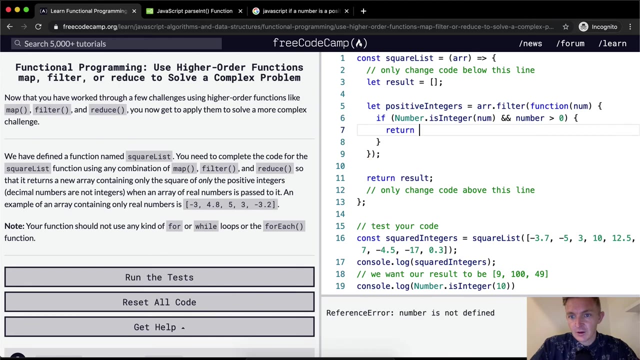 We can do both If the number is an integer And we want to pass in the number, not 10.. and number is greater than zero, Then we want to return the number And otherwise we don't. Number is not defined. 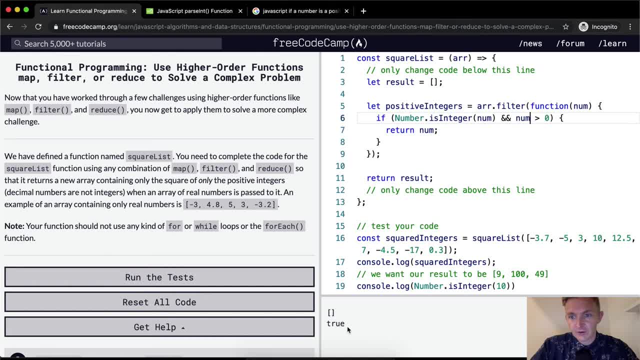 Num. It's down there I got. the error Number is not defined. Okay, So now we can get rid of this. we know what it is. Now, let's see, let's just make our. instead of returning the result, we can toss in positive integers, Okay So? 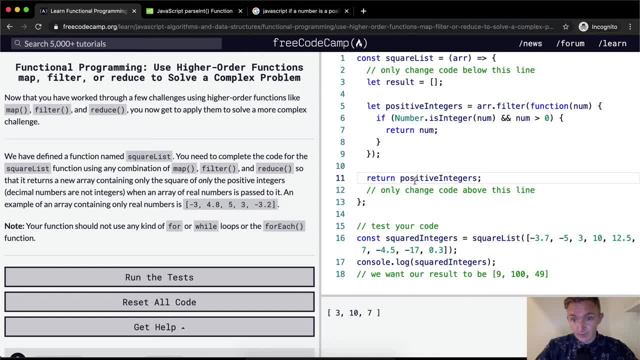 yeah, that's it, And so now all we now? okay, so now we've got all the positive integers coming out from here. Negative 5 was filtered out, but 3,, 10, and 7 all remained, And these are all derivatives of there, And so 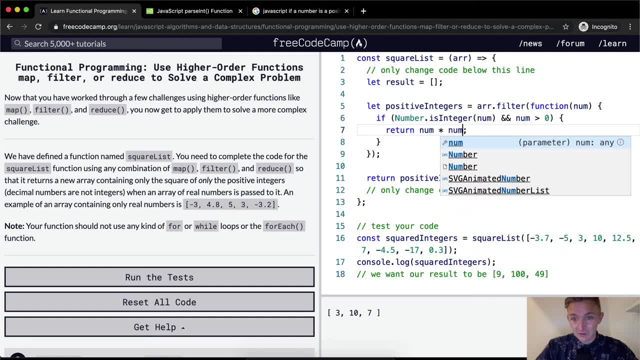 yeah, well, actually, you know, what we could do Is we can just return number times, number No, Okay cool. So now we need to map it. So let's do that. So we go. actually, positive integers squared. 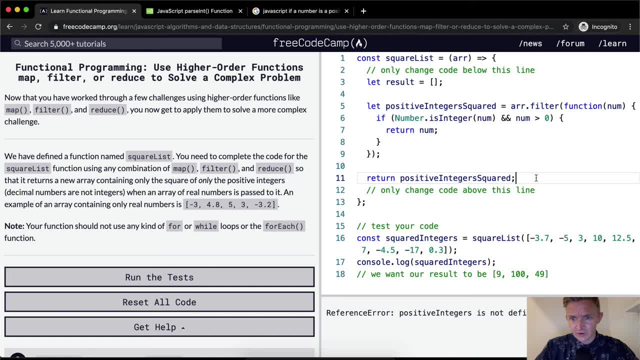 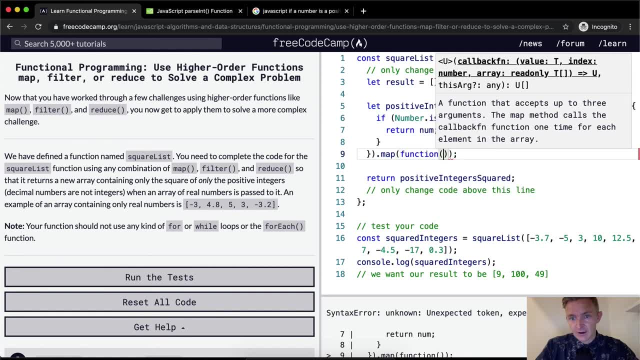 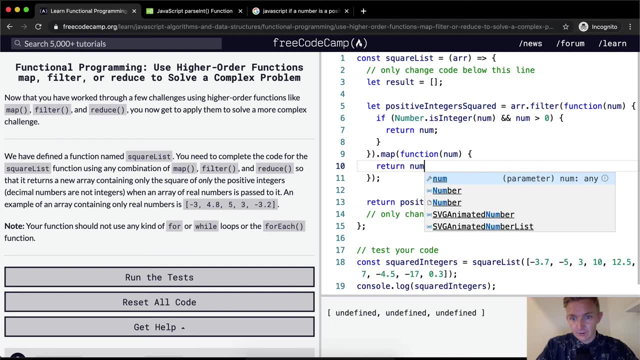 Okay, So then we return positive integers squared. We get this. What we could do now is we go dot map and we go function and the number and then we return number times number. Uh yeah, 9,, 10,, 49.. 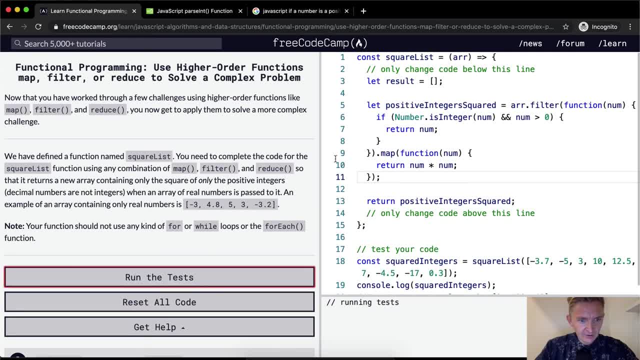 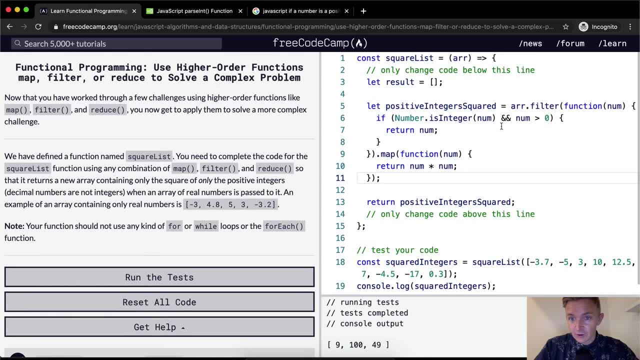 Cool. So I think that this is the right answer. We can run the test, Nice, they pass Okay. so there's probably a way to do reduce. there's probably a hundred different ways to do this. Let's do a little refactoring So. 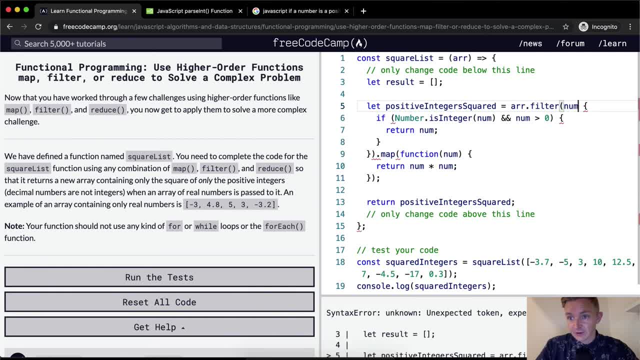 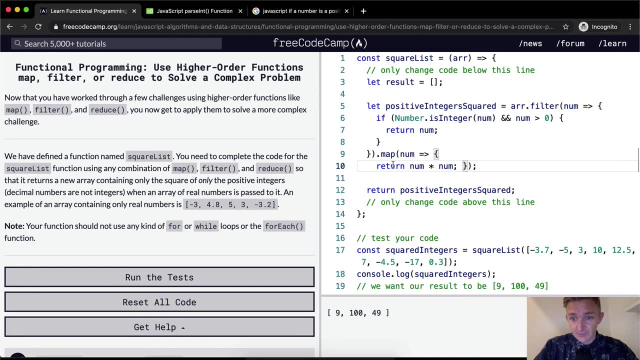 first off, this could be an arrow function and that'll make our code cleaned up a little bit more Right. This one also could be a arrow function And that cleans up our code and makes it a little more modern. This is fine to be on one line because it's so short. 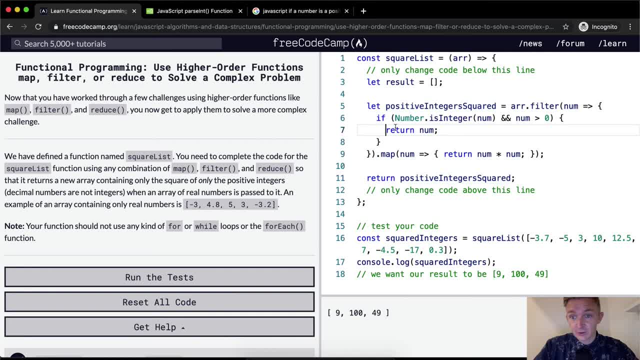 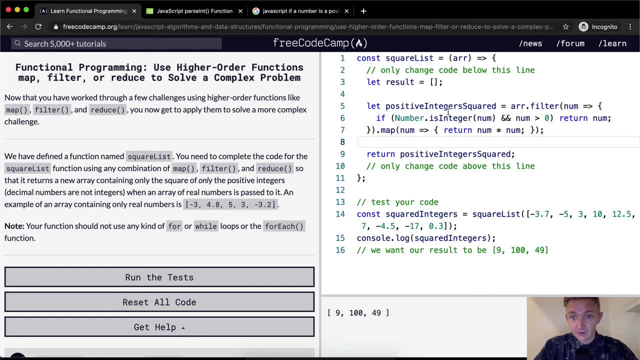 Uh, let's see here, What else could we do. This could be on one line as well, because it's short as well. So yeah, already our code's looking much more succinct, even though I'm not sure if it's as readable as it was just a little bit ago. But um, 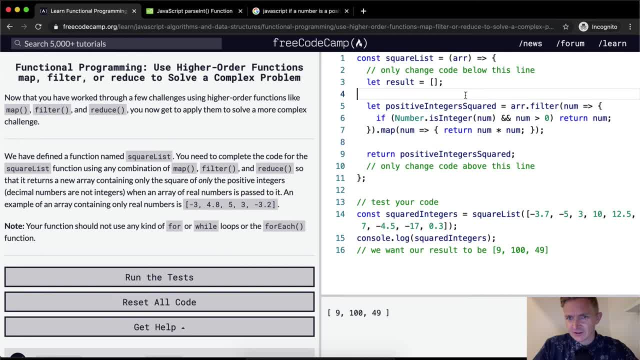 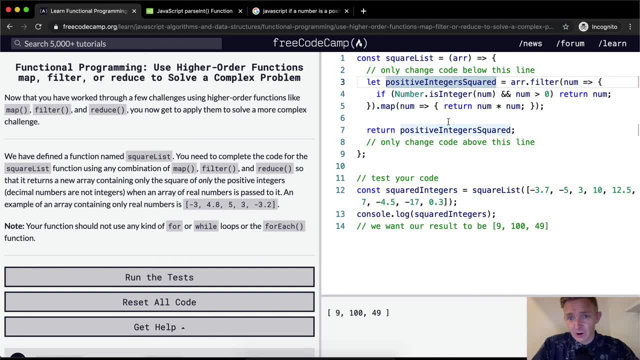 you know that's a decision that you've got to make. I guess this is. you know we don't need the result variable anymore, unless we wanted to make that, But I like naming them with. I'm a long variable name kind of guy. So if you don't like that, that's fine. A lot of this. 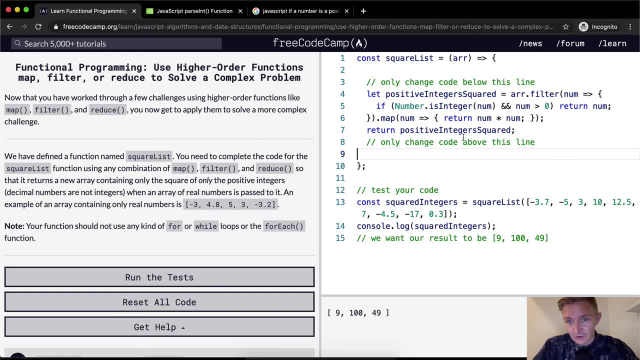 is just. this isn't necessarily the way that you have to do it or whatever. This is just how I think about it. I would probably refactor this down because positive integer squared is pretty straightforward and I would use that as a function name. 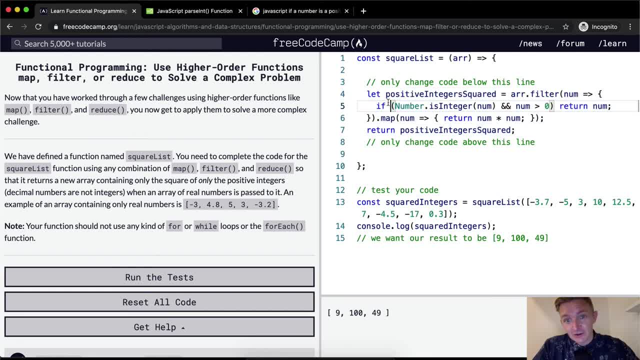 I would just basically remember that it worked in a function like this, and this is fairly readable once you get to a certain level And uh yeah, I don't see any linting errors or anything like that. This looks. it looks a little crowded. 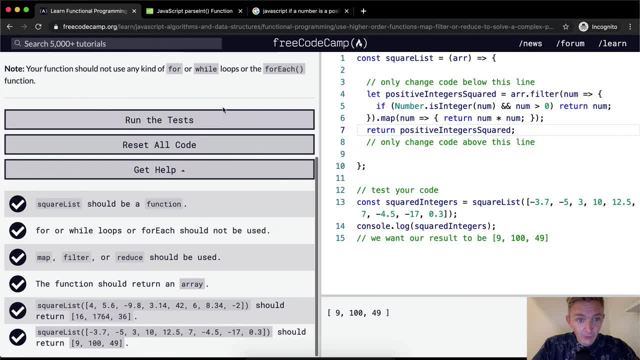 but I don't know. I think that this is good, It definitely works the way we want it to, And so, yeah, this is the refactored way of doing it. Um yeah, do you even need the brackets in here?